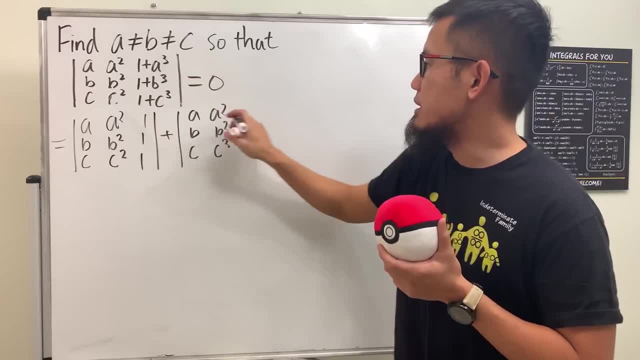 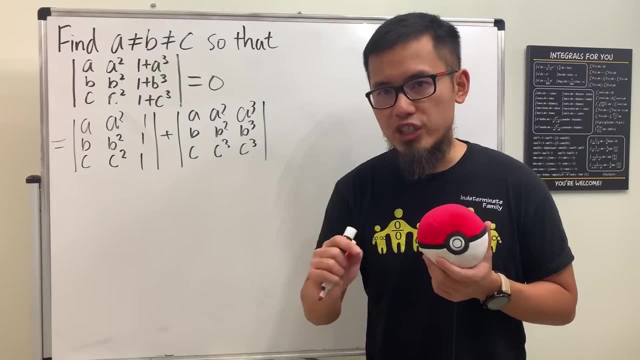 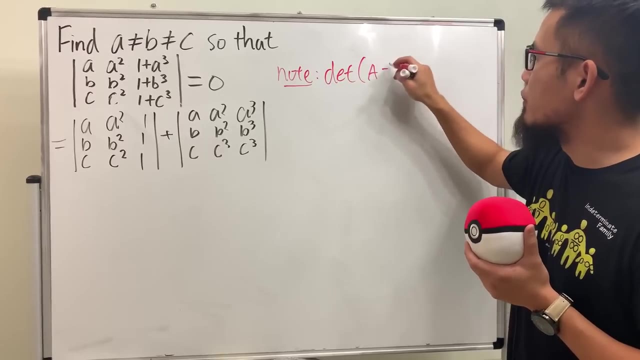 third column you have just this: a cubed, b cubed and c cubed. So this is the sum property of the determinant and this is legitimate. And let me give you guys a little warning on the side: Whenever you have the determinant of the sum of two matrix, let's say a plus b, this right here. 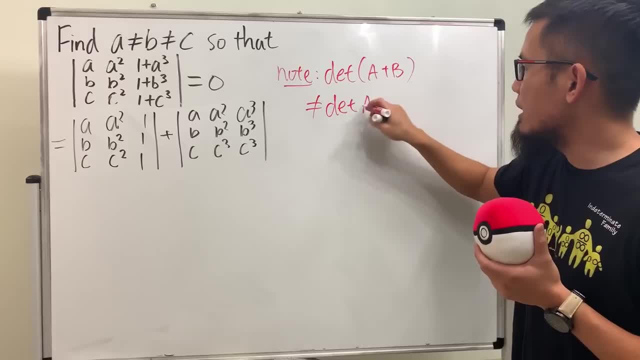 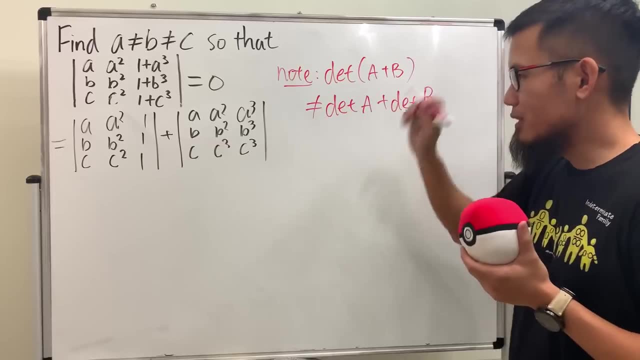 is actually not always equal to the determinant of a plus the determinant of b. Unfortunately that's not the case And perhaps, you know, do this for another video. But this is legitimate though. Now you see, here we have a. 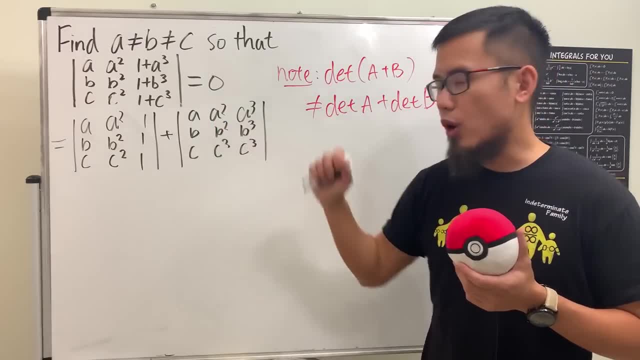 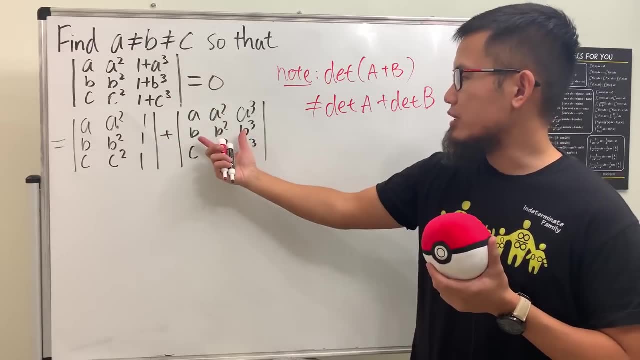 a squared a cubed. We can factor on a from this row, and when we do that, we just have to multiply the result with a. That's all. And likewise we can do the same for factoring out the b right here. 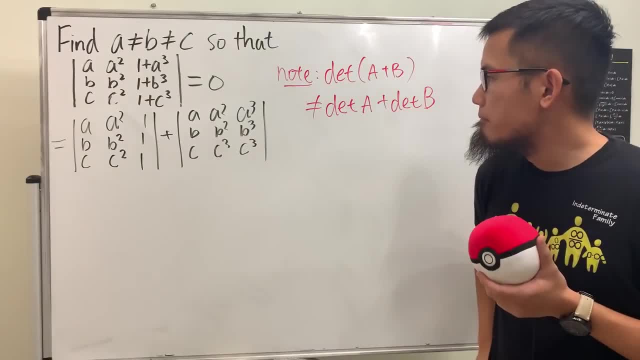 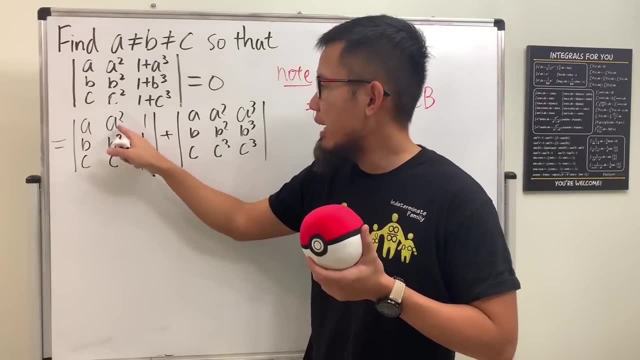 and factoring out c, So that's good. In that case, though, we will end up with 1, a and a squared, and we happen to have 1, a squared, but just at a different order, right? So we are going to do two things right here: The. 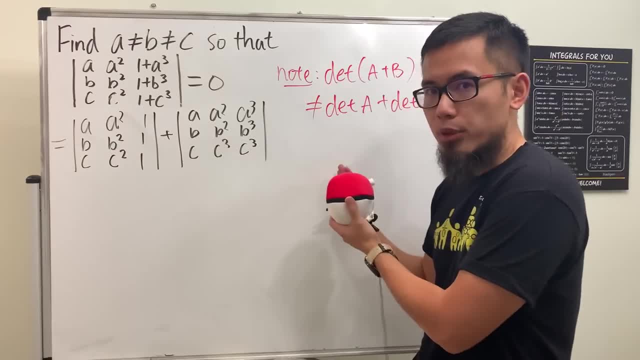 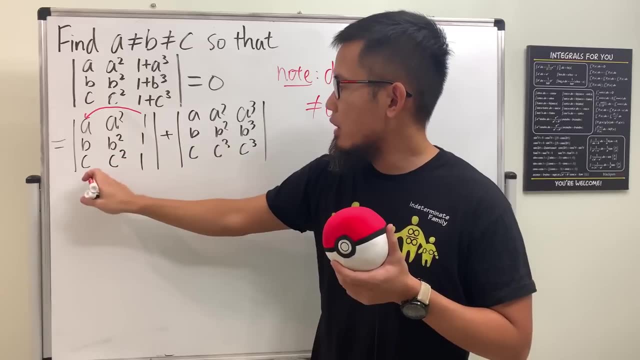 first thing is that I would like to put this into the order that we are about to get, Namely, I'm actually going to move the third column of the first matrix to the first column right here and then the first column to the third. Namely, just interchange them. We can do that. 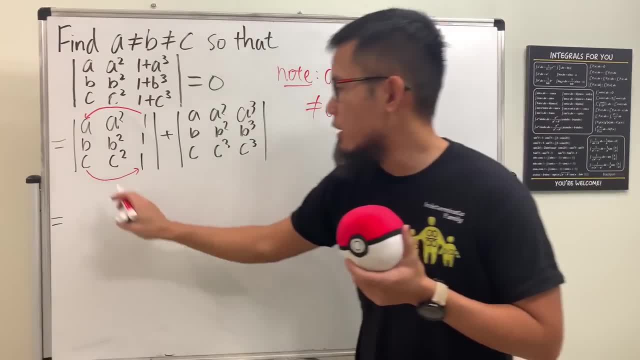 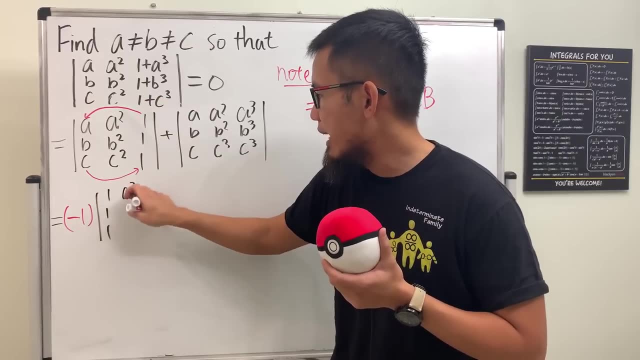 but you have to remember to multiply the result by negative 1.. So let's go ahead and do this: Negative 1 times, we will have 1,, 1,, 1, and this right here stays: a squared, b squared and c squared, and then a b, c. 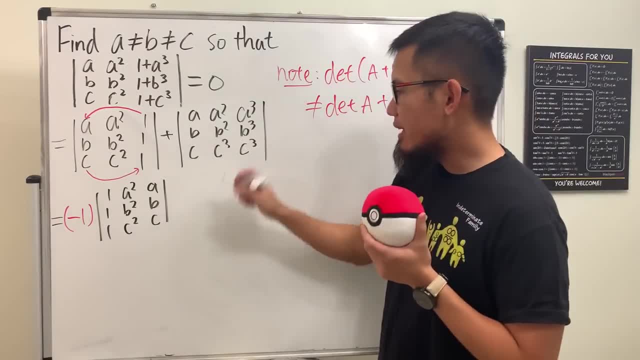 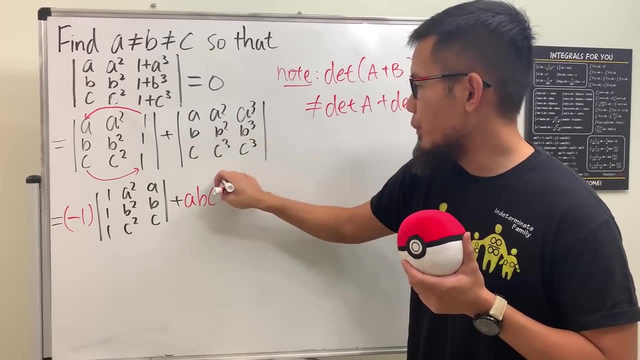 like so. So that's okay. And then for the second part, right here I'm just going to factor on a from here, and then b and c, and then we will end up with 1, a- a squared, and then 1, b- b squared. 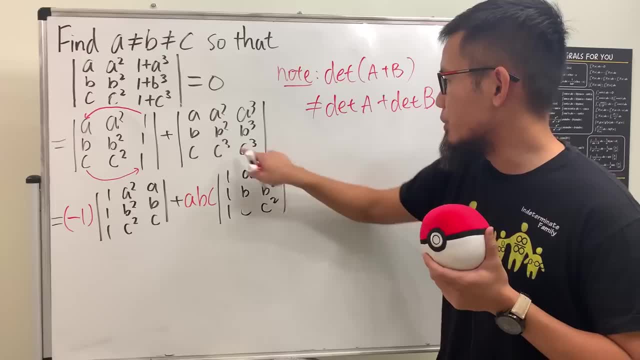 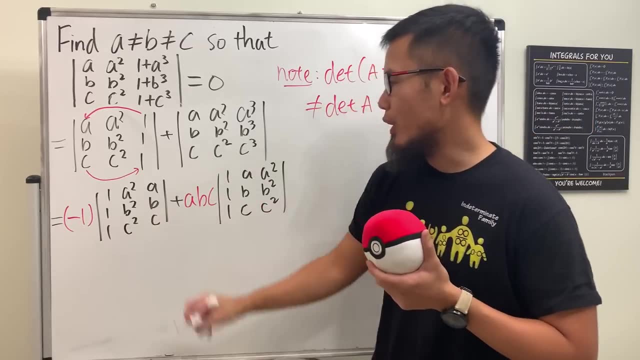 and 1, c c squared, So that's pretty good And, by the way, that's a 2. All right, So this and that they're almost the same now. Well, again, just go ahead and switch them. 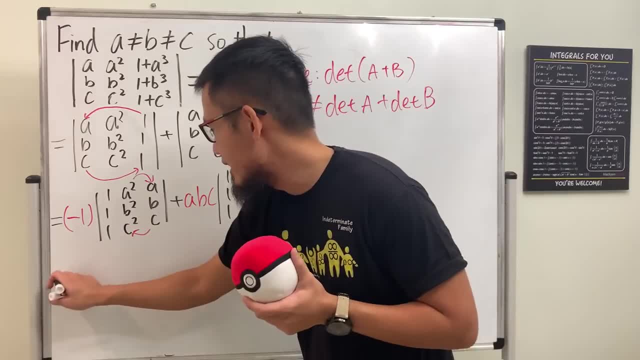 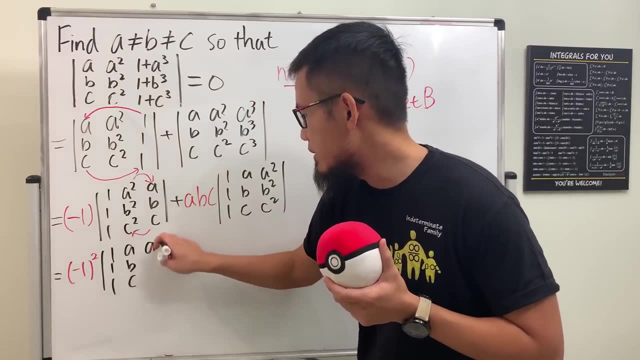 And we just have to multiply the result by negative 1 again. So we see this becomes negative 1 times negative 1, and then we have the 1, 1, 1, and then a, b, c, a squared, b squared and c squared. 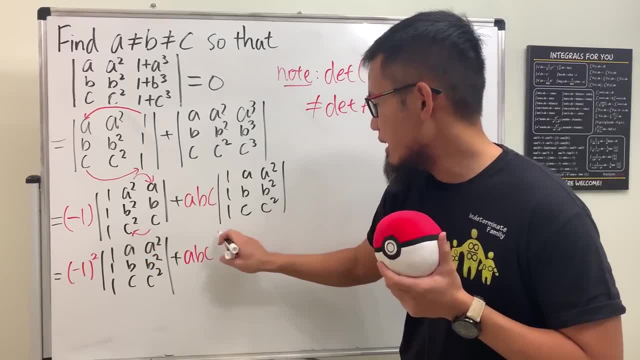 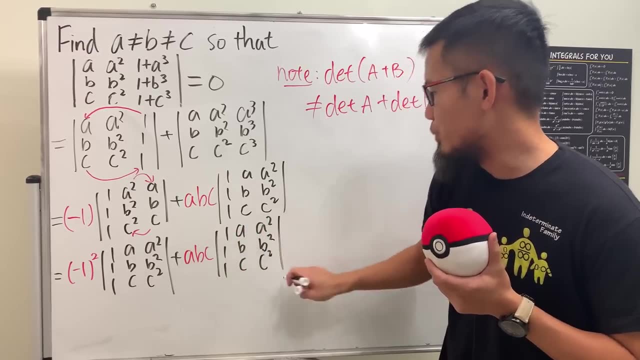 and then we just have to add it with a, b, c, and then this thing again: 1,, 1,, 1, a, b, c. a squared, b squared, c squared. I think it's pretty cool. Now, what else can we do? Well, notice that, because these 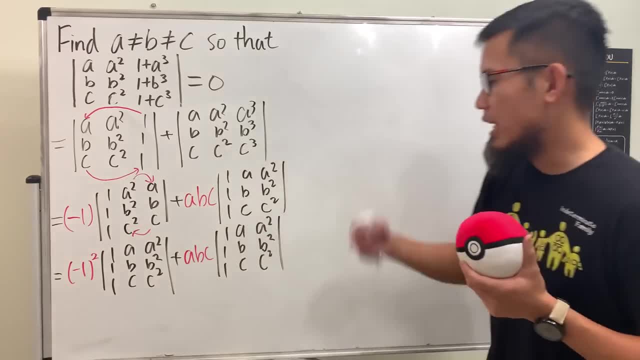 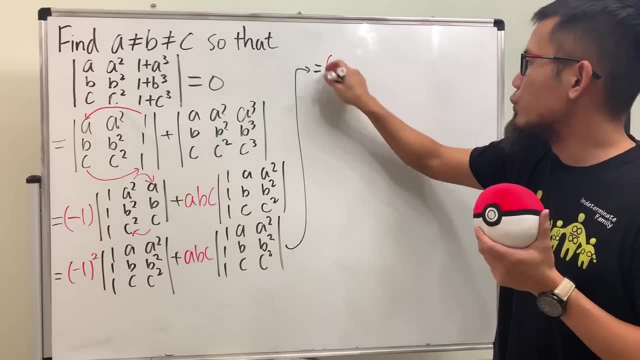 are the same and remember determinant is just a number so we can actually factor it out. So I will just put this down right here for you guys. This will be equal to. let me write this and that down first. We will have 1 plus a, b, c and then multiply by the determinant of the 1,. 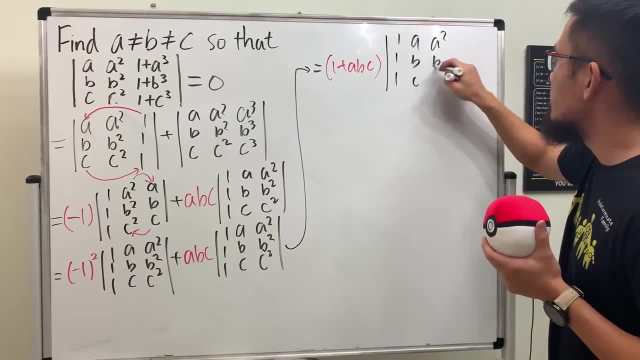 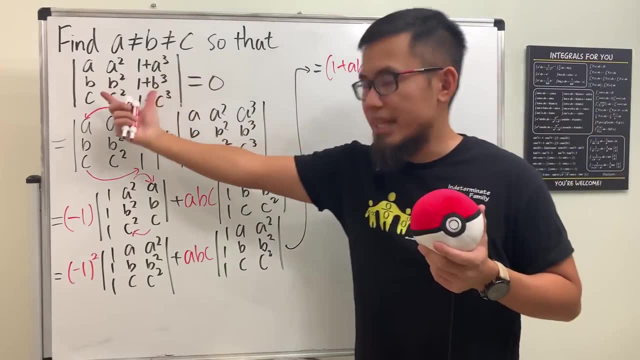 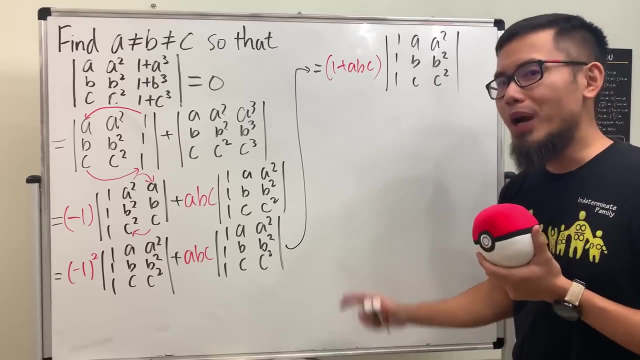 1, 1, a, b, c. a squared, b squared, c squared. Okay, this determinant is easier to compute than that determinant, But this is still not the best. The best one that we like is the one that has a lot of zeros, right, So we are going to do some. 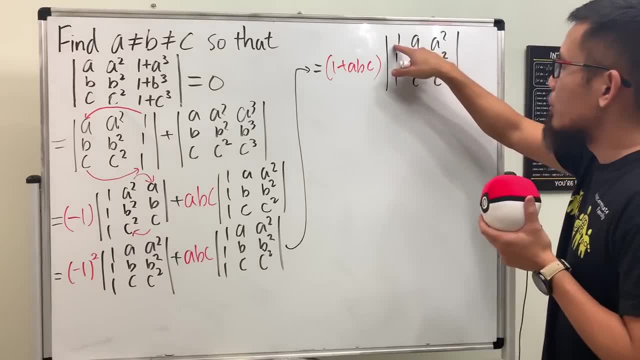 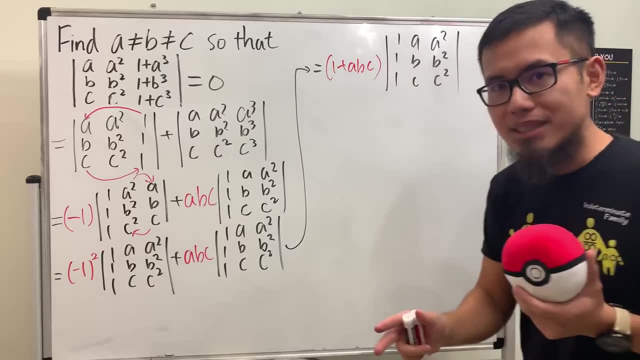 rule reduction here, And what we can do is we can multiply this by negative 1 and add it to the second row, so we can put the zero right there, And when we do that, the truth is the determinant stays the same. So that's so wonderful, right? So we can just do some rule operations. 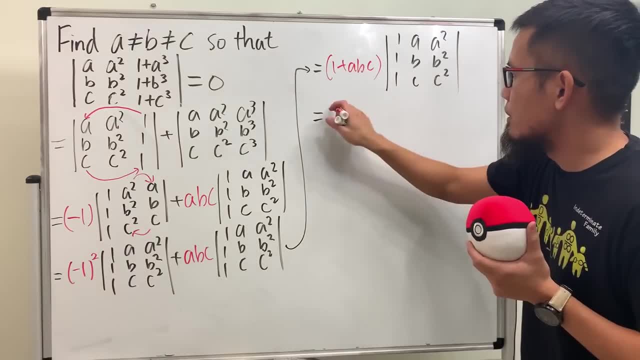 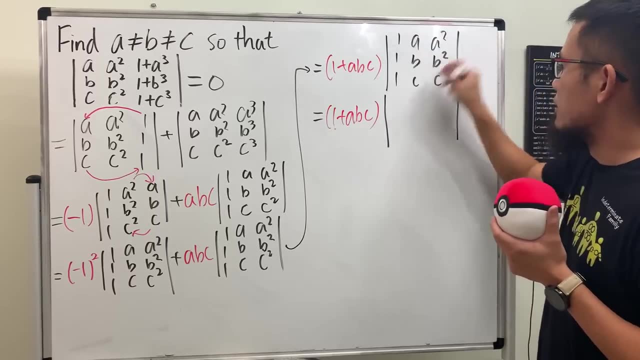 right here. So I will just keep the 1 plus a, b, c in the front and then I will just write this down for you guys. The first one stays and then rule reduce: we get zero and then this becomes negative. 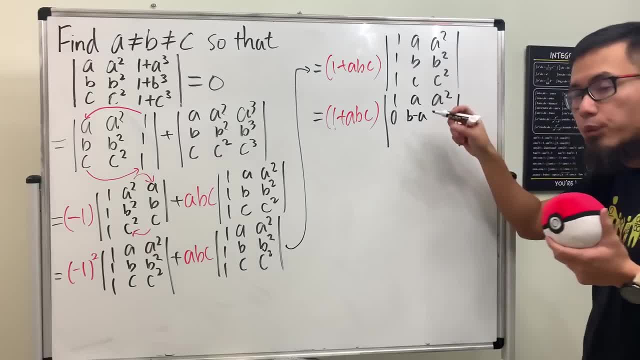 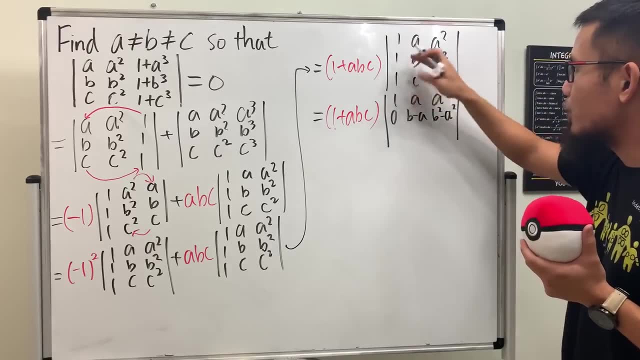 a plus b. I'll write it as b minus a, And then we have b squared minus a squared. And since we can do this to here, why don't we do it to the third row as well? So multiply this by negative 1,. 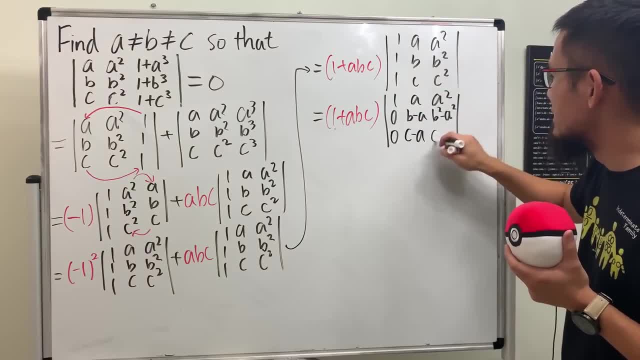 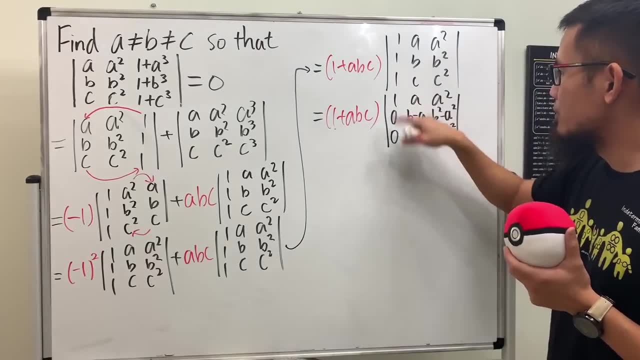 and add it here, We get zero c minus a, and then c squared minus a squared. Very nice, right? And now you can do the expansion right here and you'll just end up with a determinant of the 2 by 2 matrix. 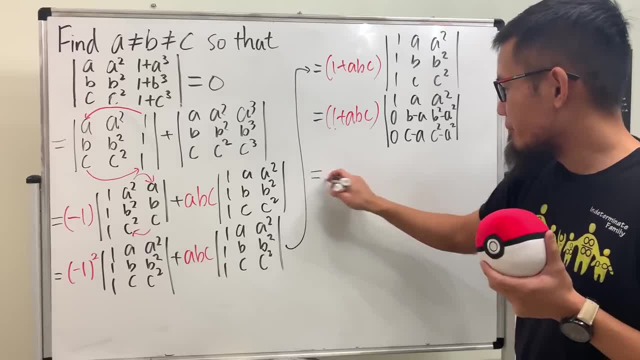 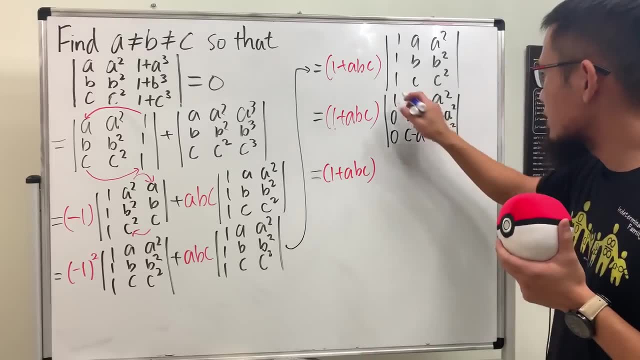 which is much better in my opinion. So we'll do that. So here I will still keep the 1 plus a, b, c here, and then just kind of ignore this, ignore that, And this is a positive 1. Remember. 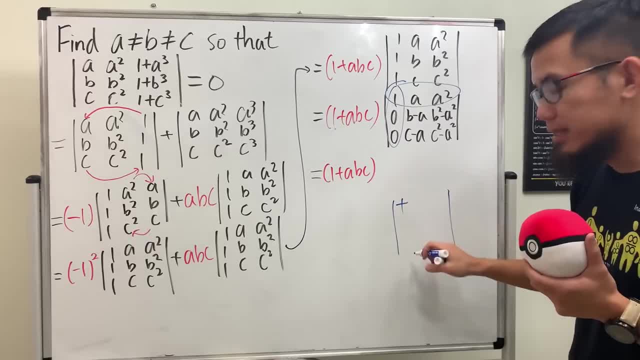 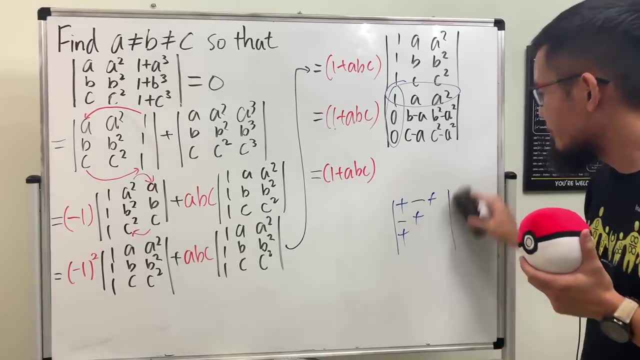 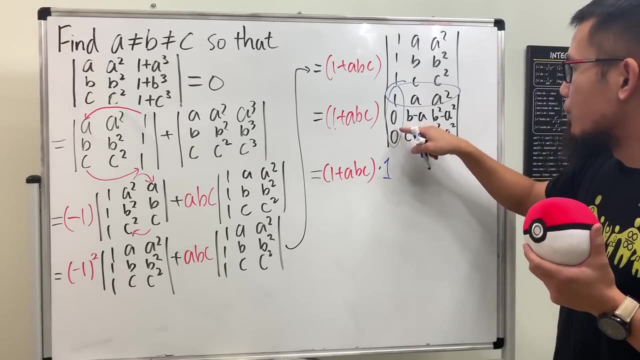 you do the expansion, you have to pay attention to the sign. Start with plus and then minus, minus, and then plus, plus, plus, And the sign just alternates right. So if you do the expansion right here you keep the positive 1.. And the beauty is that. well, actually, because of zero, 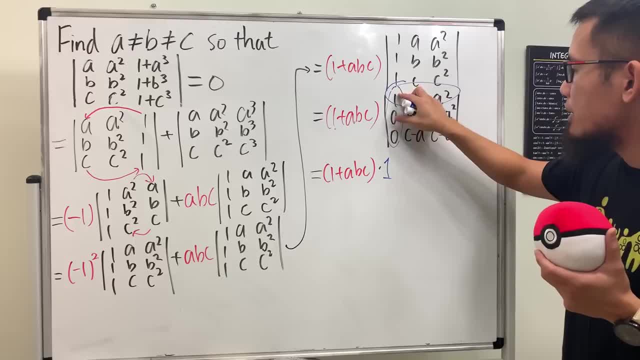 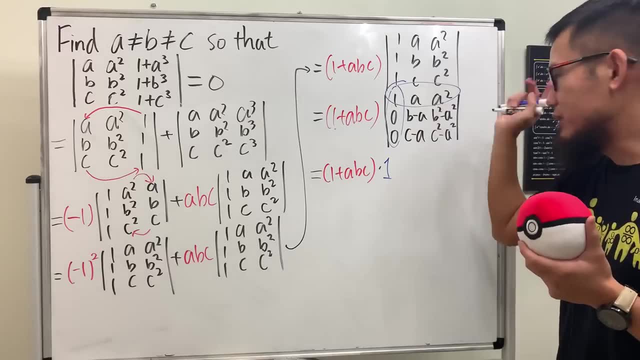 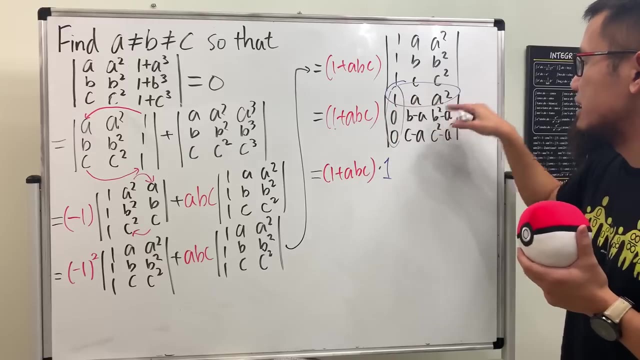 so you can just ignore that. It's technically 1, right times this, And then you add it with zero times the matrix of this, this, that, that, that. So whenever you have zero in your row or column, you can just do: delete this, delete that. 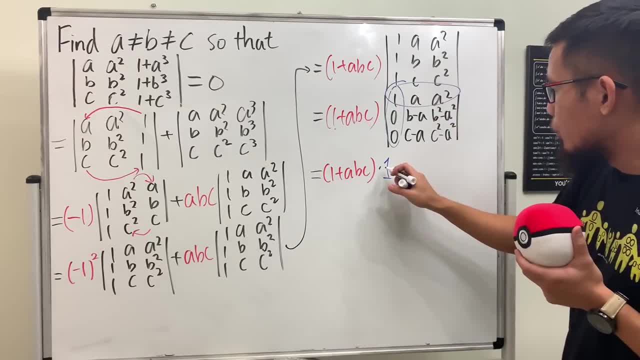 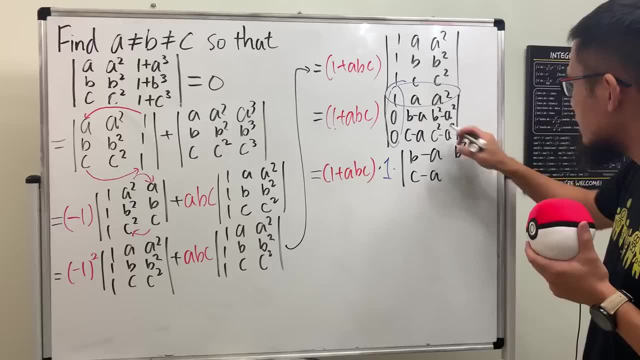 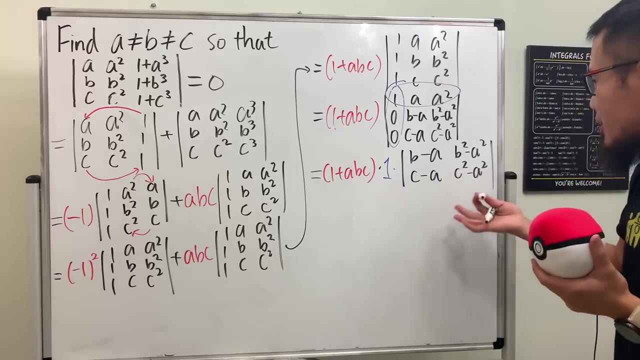 and then just focus on the rest. So that's what I'm doing, All right. so 1 times the determinant of this: b minus a, c minus a, and then this is b squared minus a squared, c squared minus a squared. Perfect. Now what else can we do? Don't be lazy. Now just go ahead and compute the. 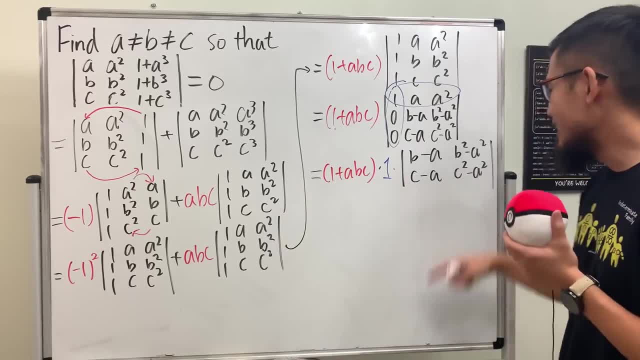 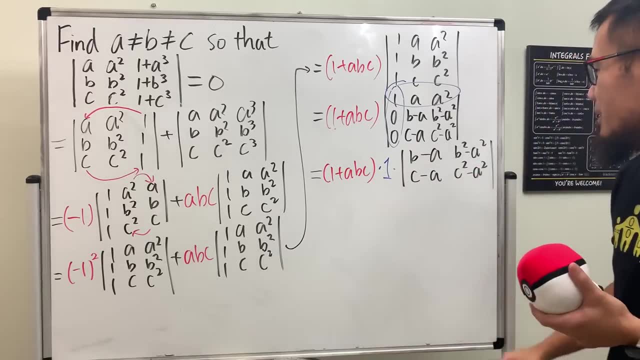 determinant of this, And if you really want to do some factoring business, you can look at this as b minus a times b plus a and the factor of b minus a, But I think we should be okay, Yeah. Anyway, though, I'm just going to write this down, We have 1 plus a, b, c. 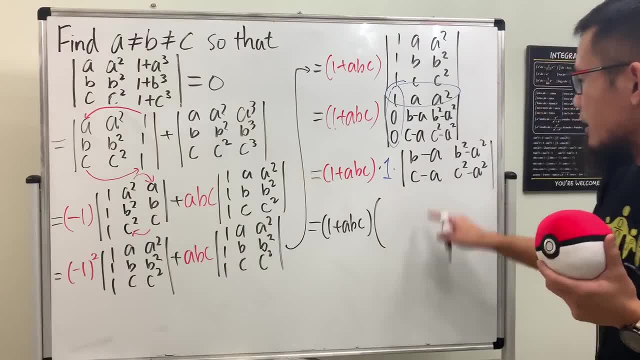 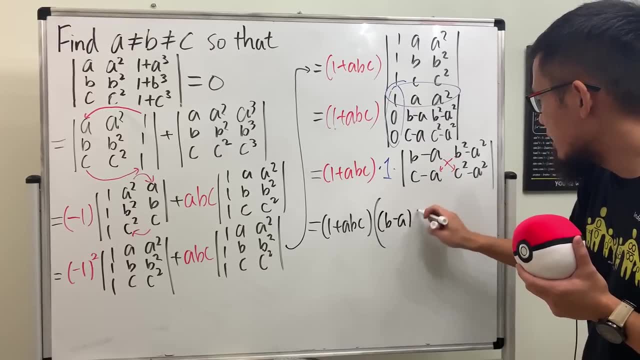 times 1, doesn't matter, And the determinant of this guy is just this times this and then subtract this times that. Pretty easy right. So we will have b minus a c squared minus a squared, and then we have to minus. 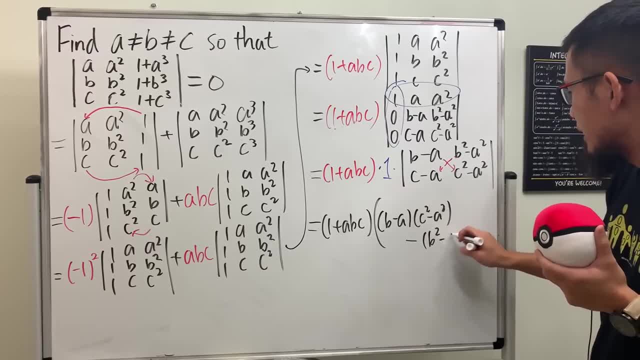 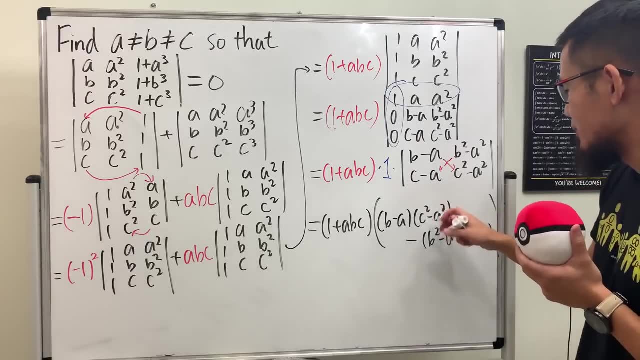 b. c squared minus a. squared times c minus a, like this: All right, So now, as I told you, we can factor and just do the algebra. This right here is c minus a, c plus a, and this right here is: 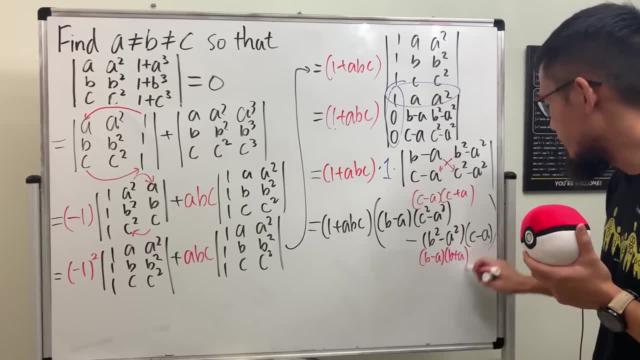 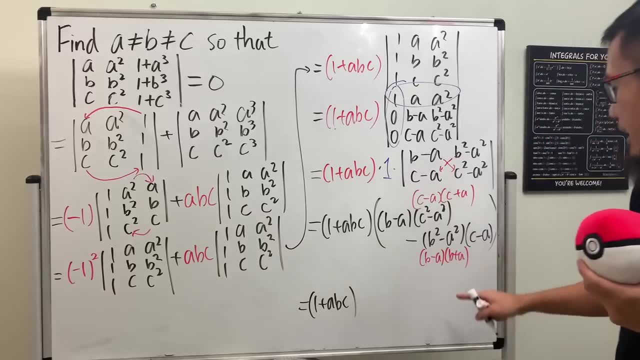 b minus a and b plus a. So let's see what do we really have? All in all, we have 1 plus a, b, c, and then from here we can factor out b minus a. So that's nice. So we have the b minus a. 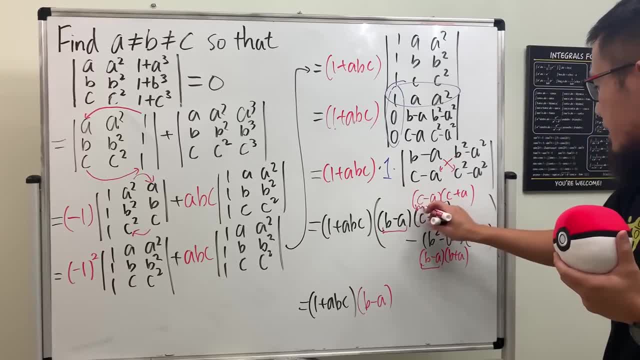 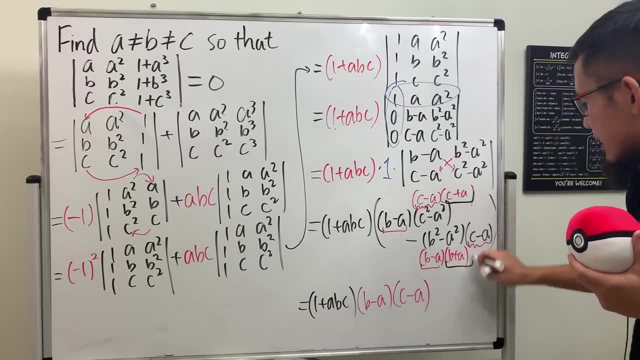 and then we have c minus a, c minus a. So go ahead and do that. And lastly, we have this minus that inside of the parentheses. So here we have c plus a minus b plus a, like so, And this right here. 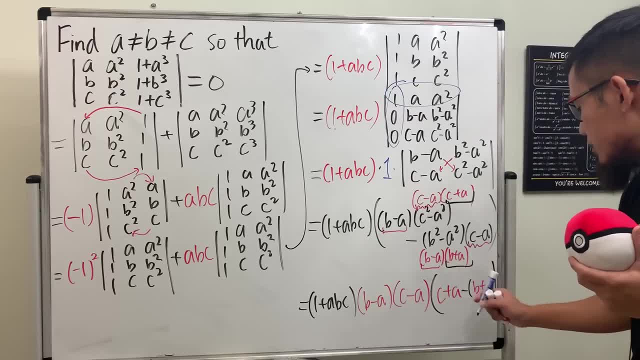 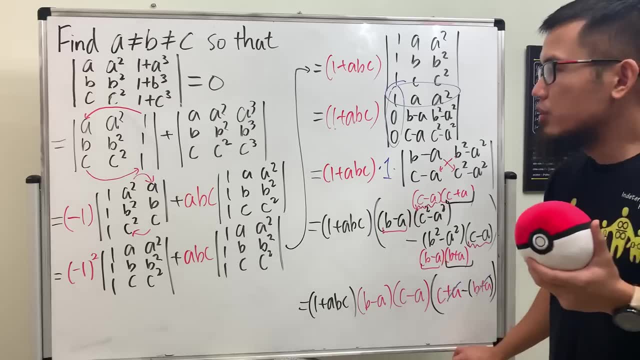 we can simplify it. You see, the a minus a is just 0, so of course this and that will be out. So the last parentheses is just nicely equal to c minus b. So all in all we can come back here after all the simplification. 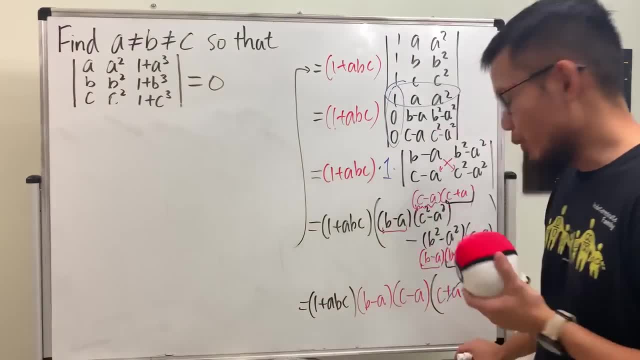 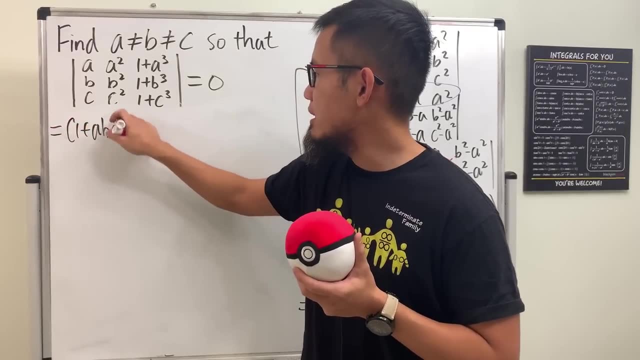 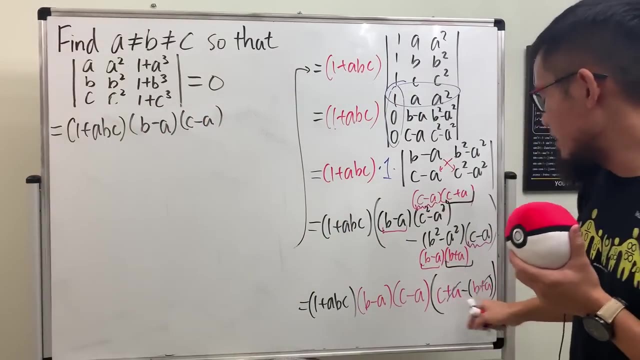 Magic. pretty much, You can just erase all the work and just tell people that, hey, you know what? The determinant of this guy is just nicely equal to 1 plus a, b, c times b minus a, c minus a, and then we also have c minus b. 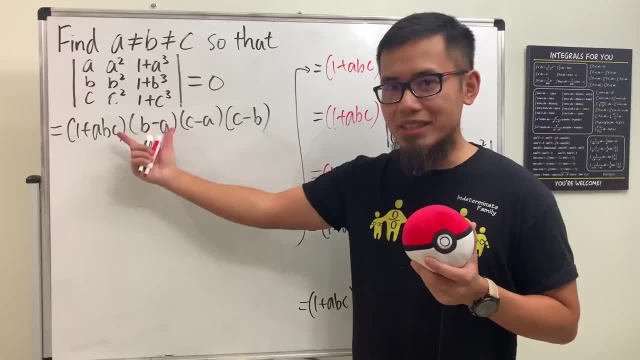 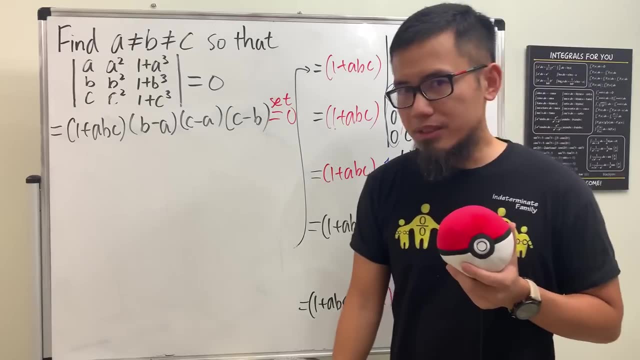 Pretty good, Now remember we want this to end up to be 0. So we are going to set this to be equal to 0. And here is the time that we are going to use our condition. Notice that a is not equal. 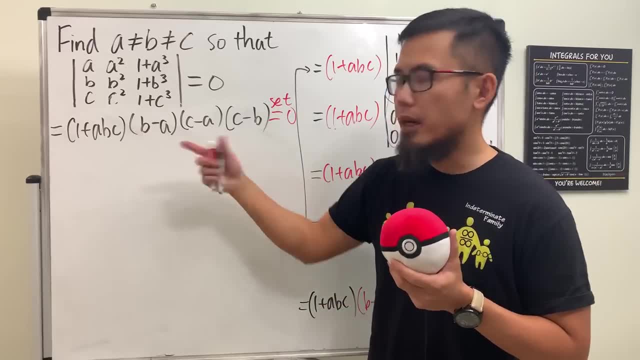 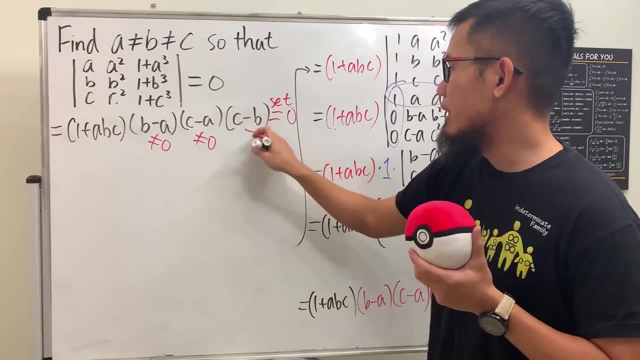 to b is not equal to c, so that of course a and b are not equal. That means this right here cannot produce a 0.. Likewise, this factor cannot be giving you 0.. Likewise, this cannot give you 0 neither. So how can we conclude? 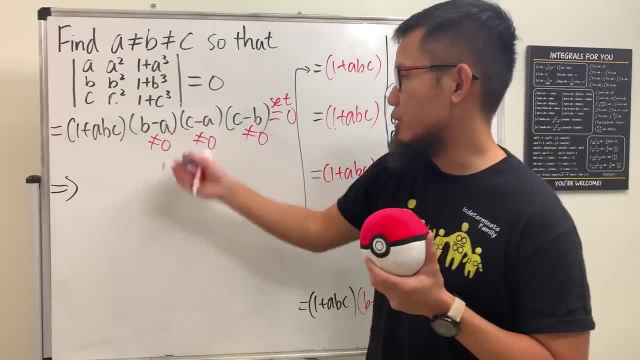 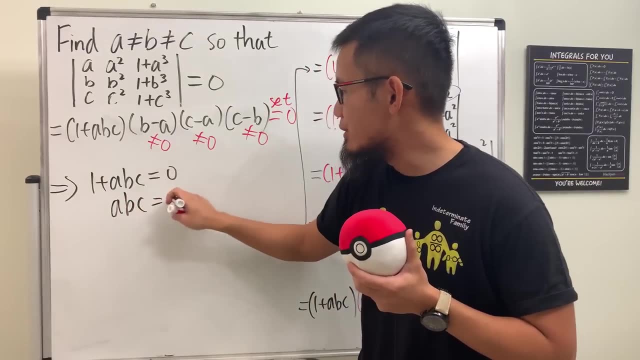 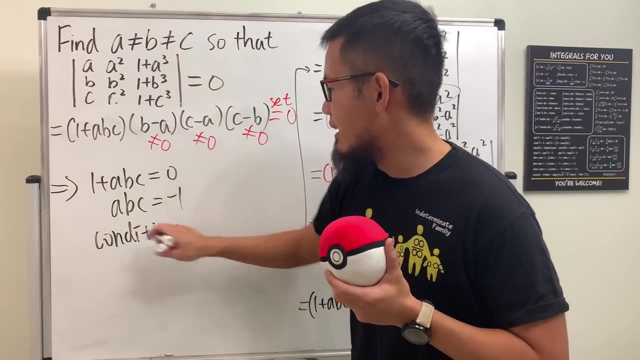 So the only hope for us to end up with 0 is that 1 plus a, b, c has to be equal to 0. Namely, a b, c has to get to negative 1.. So this, right here, is the condition. That's pretty much it. 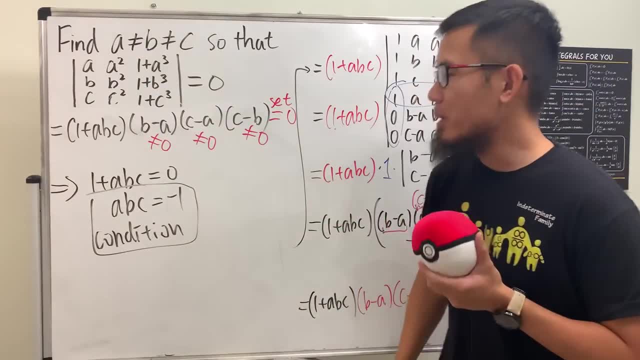 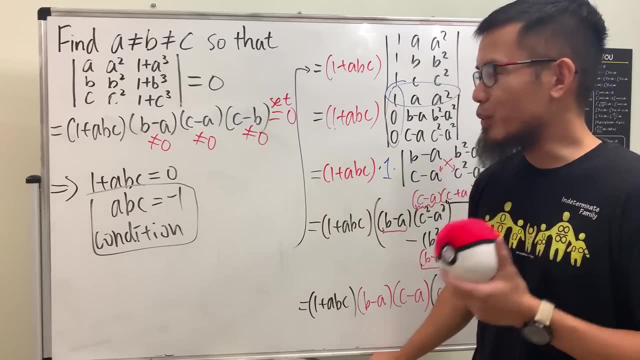 So if you want to produce a matrix in this particular form, all you have to make sure that is: a times b times c is equal to negative 1, then this right here will be it, And of course you have infinitely many choices for that. 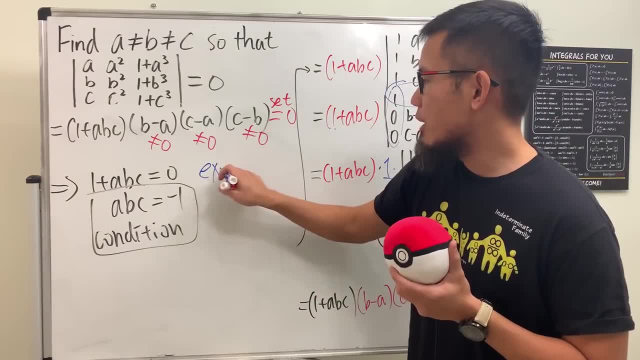 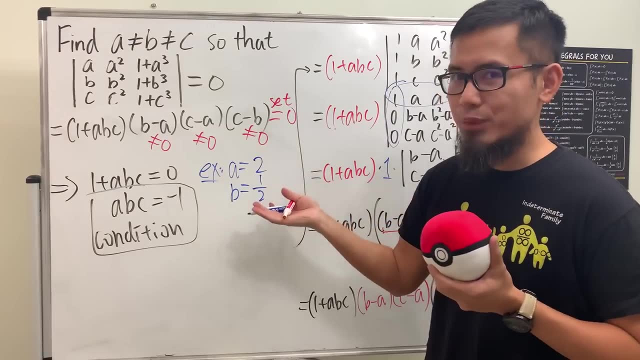 Let me just give you guys a quick example So you can take a to b. Let me not be too creative. I'll just say two b is equal to one half, so we get positive 1. so far I need to end up with. 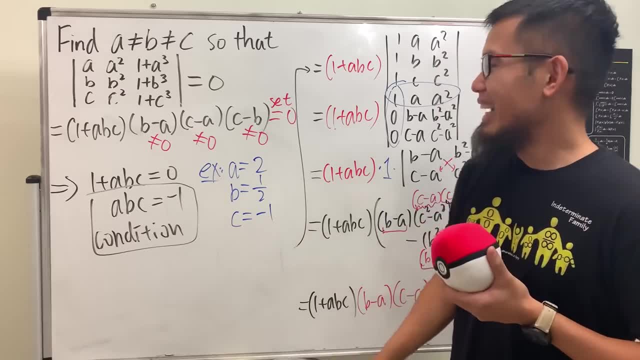 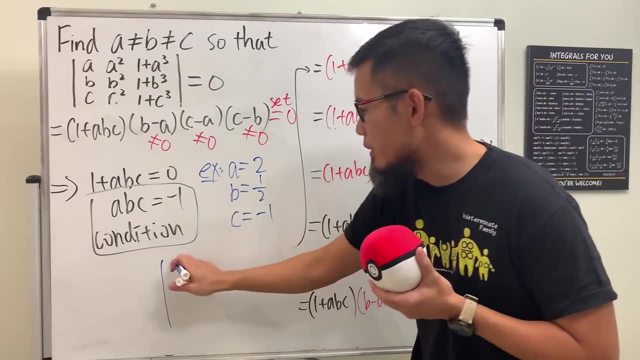 negative 1, so c is equal to negative 1 there. okay, And then just plug in, Then you will see that. Let me tell you: we have 2 squared plus 2 to the third power, so we get 2 4 9.. And then put: